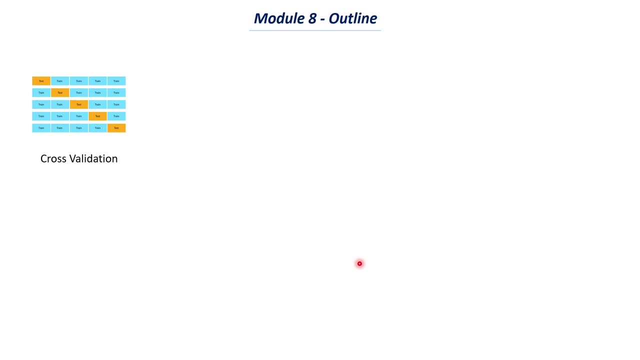 So, once we understand about cross-validation, we will also be discussing something called a scaffold cross-validation, So how to implement this scaffold cross-validation in Python. So this is the first topic, and the next topic will be on hyperparameter tuning. So, again, this is one of the most important things that we have to do while implementing a machine learning model. 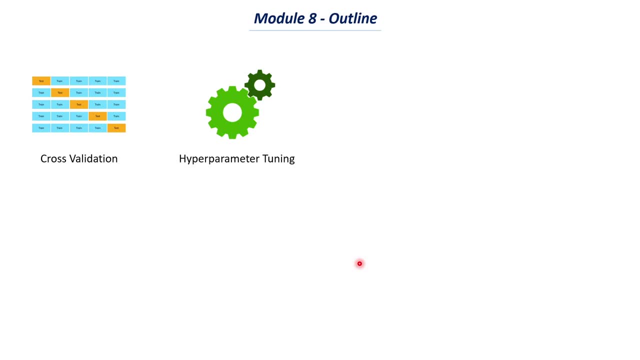 So in machine learning we usually have two kinds of parameters. So first kind of parameter is the model parameters, and these model parameters are derived from the data set that we have. So if we think about a linear regression model, we have the parameters such as m and c, where m is our slope and c is our intercept. 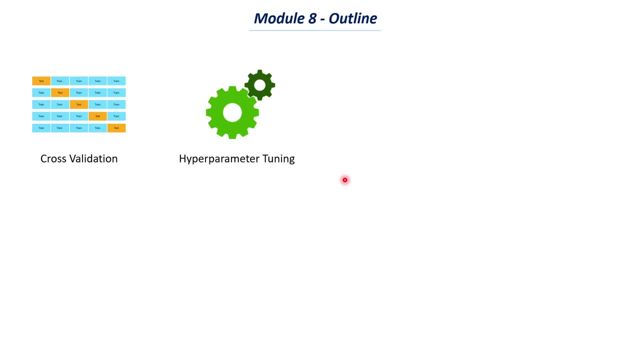 so m and c values are derived from the data set that we have, and the other set of parameters is called as the hyper parameter, and this hyper parameter determines how your model is being trained. so we change these hyper parameter values in order to get the best fit of the model in order. 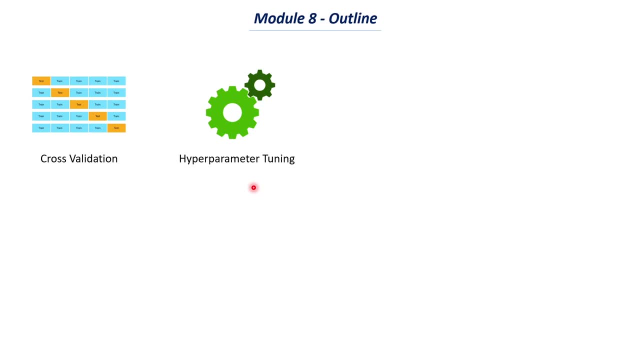 to get an efficient model. so we will be discussing about what is this hyper parameter tuning and how we can implement this. okay, and when we talk about hyper parameter tuning, there are two main important techniques that we can work on, which is grid search cv and randomized search cv. so this 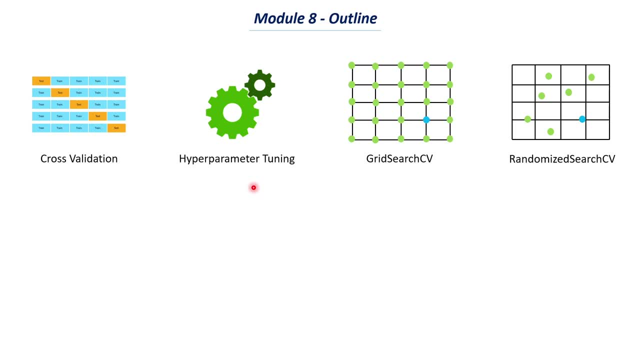 will be the next set of videos that we will be discussing. so first i'll explain you what is meant by this grid search cv and randomized search cv, and we will be taking an example and working on python in order to implement this grid search cv and randomized search cv. okay, and one more thing. 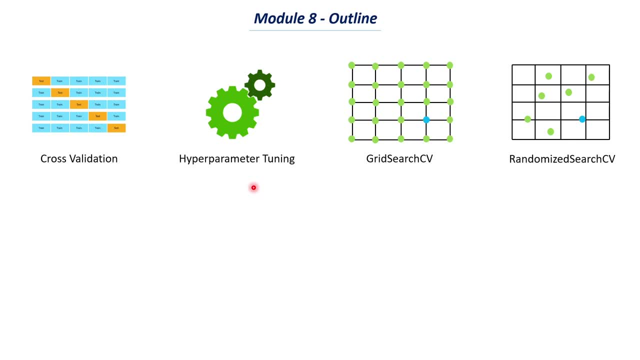 that i wanted to mention. that is like in all the videos, there will be both theoretical aspects and and so on, but so if we think about cross validation or hyper parameter tuning, in the first part of the video, i will be giving you a theoretical aspect of all. 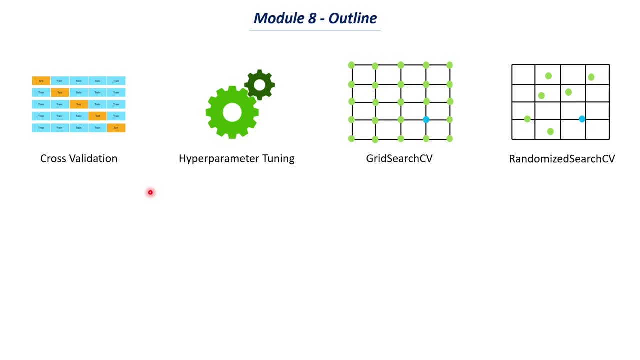 the concepts that is present there and, based on that understanding, we will be implementing the same thing in python. so this would be the structure of the upcoming videos in this particular module. so once we complete this- cross validation, hyper parameter tuning, grid search cv and randomized search cv- so using all these things, we will be discussing how to select models. so the next topic. 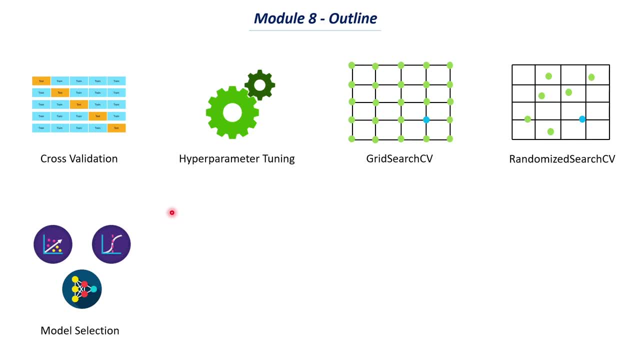 will be on model selection. again, this will be both conceptual and anson part will be covered here. so, using all these techniques, we will try to, you know, select the best model which is suitable for our particular problem. so once we complete this model selection, the next part will be on model. 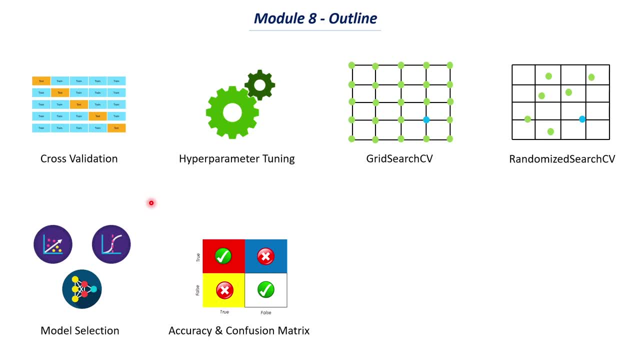 evaluation. so, under model evaluation, the first thing that we'll be discussing is accuracy and confusion matrix. so we'll be discussing in detail about what is this: accuracy, accuracy scores and especially confusion matrix. so these are all very important metrics when it comes to classification problems in machine learning. okay, so the next topic will be on. 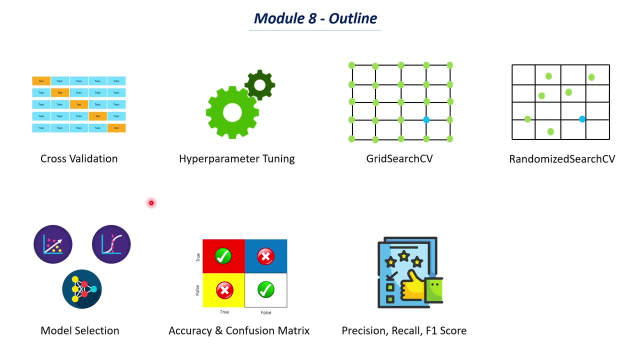 precision, recall and f1 score. so there has been a lot of ambiguity on this particular topic, and this is also used in our classification problems, where these are again evaluation metrics which are more reliable when compared to the accuracy score. so we'll be discussing about what is meant. 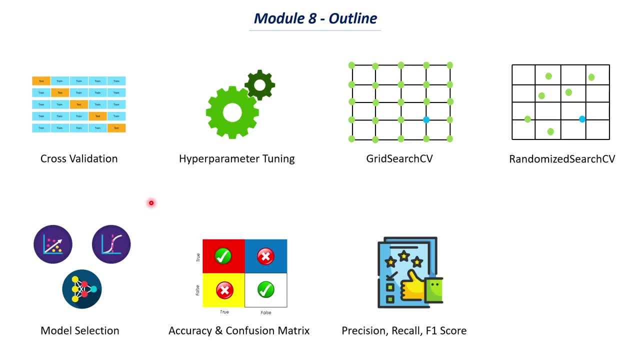 by this precision, recall and f1 score and how to calculate this while we are working on a ml project, so we'll be discussing this in python as well, and the last part of this module 8 will be metrics for regression. so we know that we have different error metrics, such as mean, absolute. 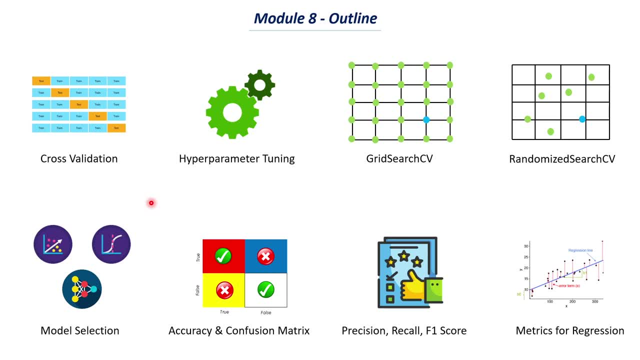 error, which is called as mae, and also we have mean squared error and etc. right, so we will be discussing what is meant by each of these error metrics and what is the significance of each of these error metrics. so these are all the topics that will be covered in this particular module. 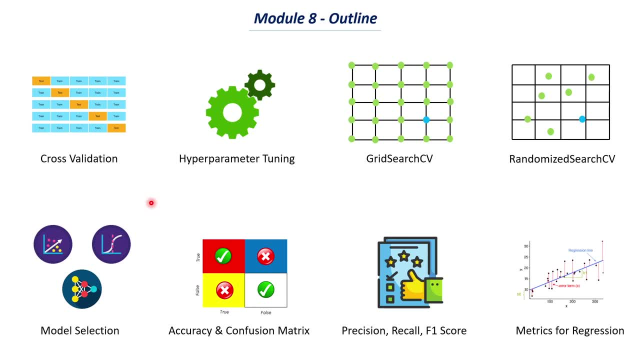 and i hope that most of you know the importance of all these modules. okay, so all these topics. so so first, as i've told you, the first part will be cross validation and hyper parameter tuning and model selection, and the next part will be on a model evaluation for both classification.